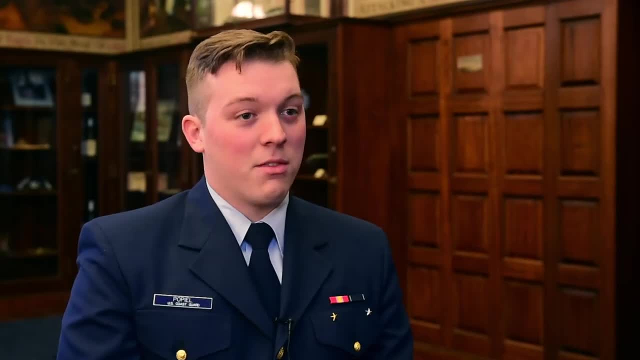 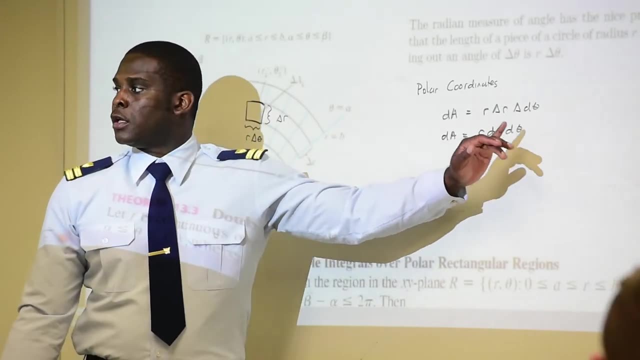 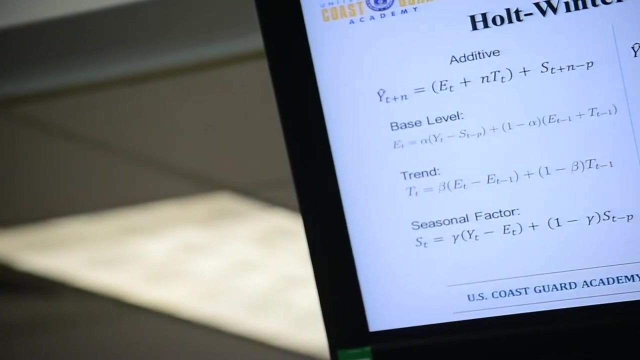 different way, then that's the major for you. ORCA is the math major at the Coast Guard Academy, but it really goes beyond that. The ORCA major is all about using math to solve complex problems. I like computer science, I like math. I kind of like projects and thinking about those types of problems. Once I figured that out. 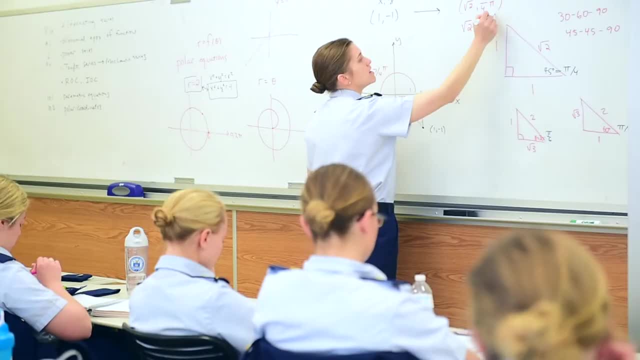 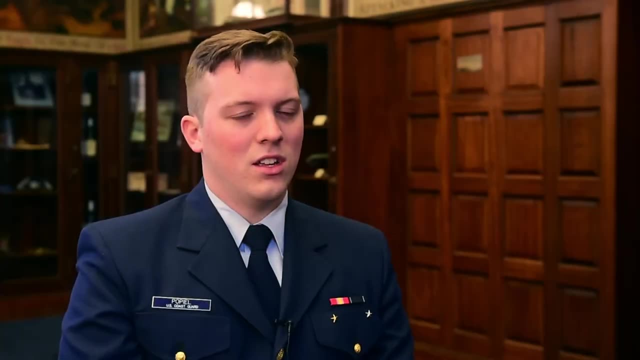 that's when I knew that I thought ORCA was for me. Math isn't always the easiest subject, as I'm sure a lot of people know, but the faculty is fantastic and they make themselves available. So your biggest challenge almost turns into your biggest triumph, because once you finally get a concept down or you figure out how to do a problem or how to do a process, 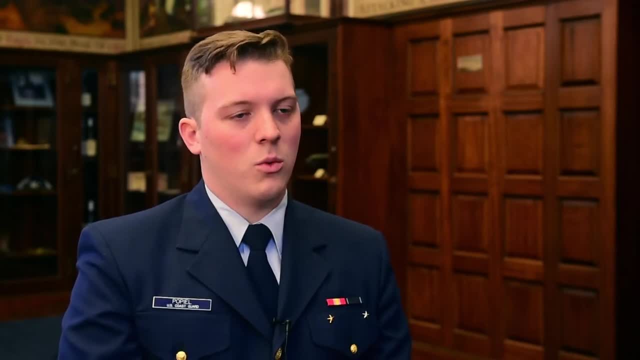 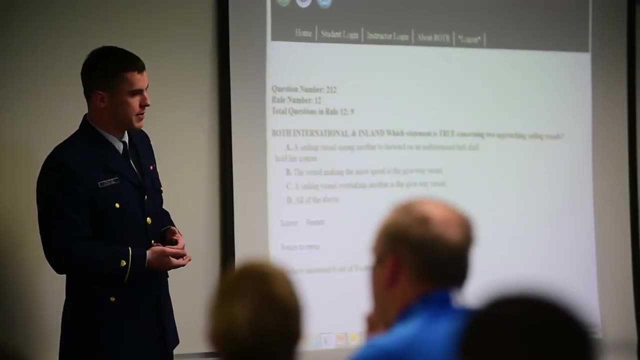 you just feel that accomplishment, that sense of pride in what you've done and the work that you've put in. We actually get to do a project that is relevant to what is going on in the fleet right now and, depending on the outcome of that project, 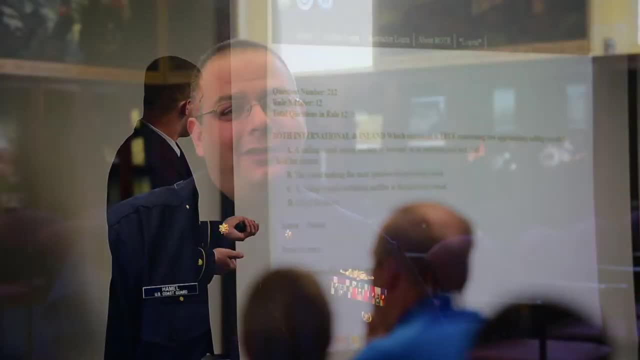 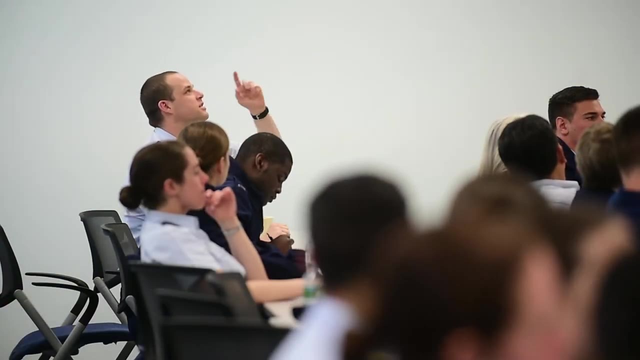 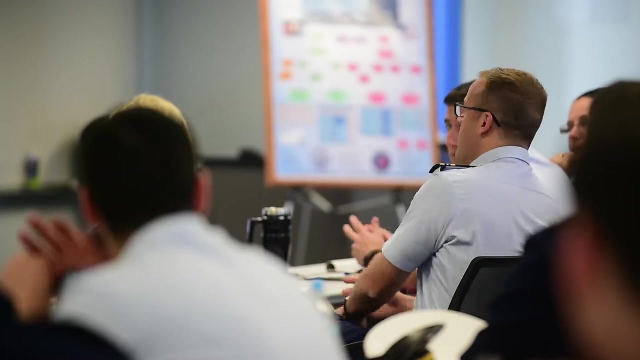 could even be applied to solving that problem in the fleet, OR majors are really involved in real business cases from the Coast Guard. so we're sought out by operational commanders to do projects to basically take the bigger data, the bigger decisions that require analysis and give them the tools to make best decisions. 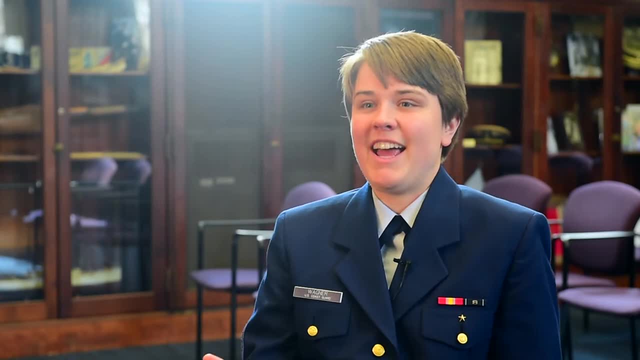 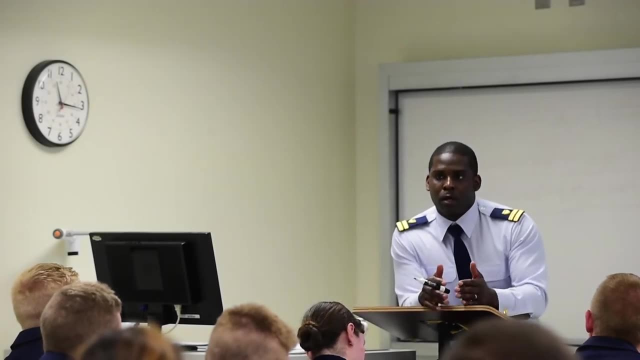 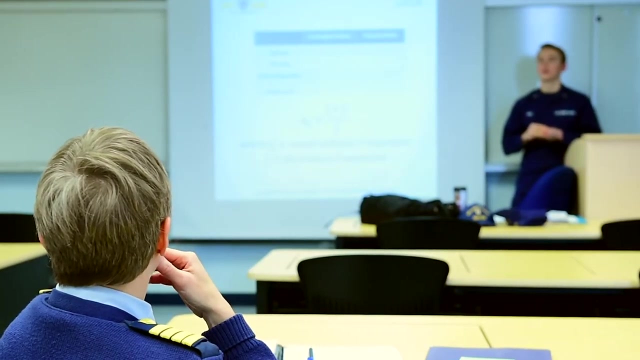 So I think it's really neat to be like: all right, I'm actually solving this problem because someone has this problem for real and they need help with it. Overall, it's definitely the analytical thought process that we're aiming for. We want you to leave here being able to at least understand how to frame a problem, understand what tools you have in your bag to solve it. 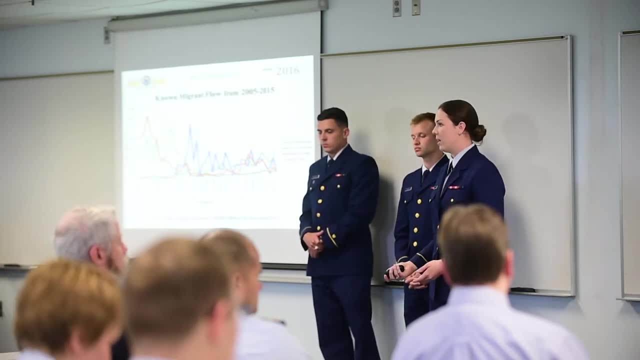 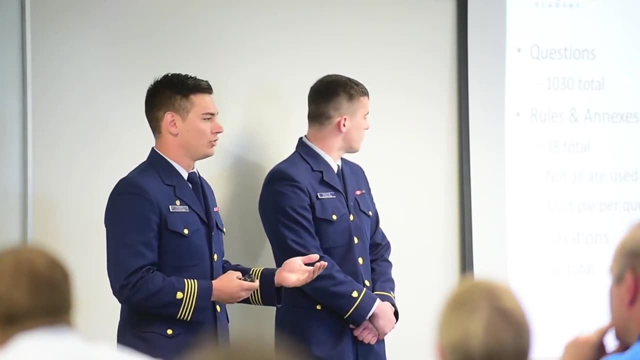 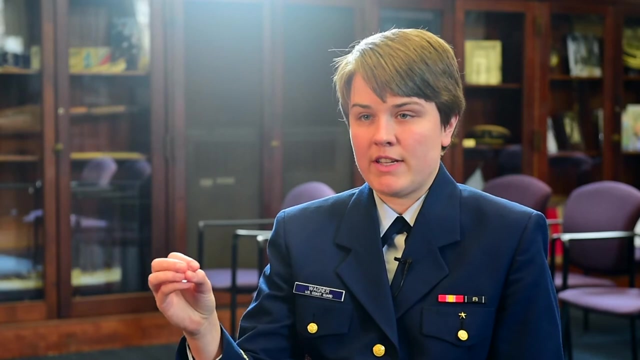 know how to ask the appropriate questions to get the information you need in order to attack that problem and just to be generally aware of where you can apply what we've taught here to other issues that you may see in the fleet. You get this. you know people out in the fleet and they're saying: we have this problem and we're not sure how to fix it. can you help us with it? 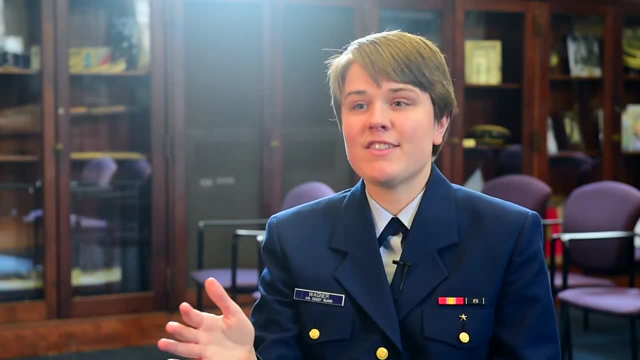 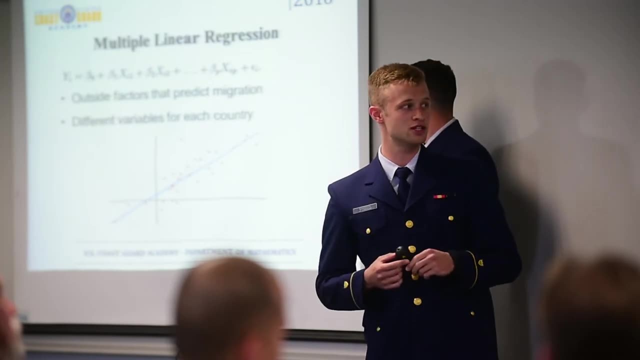 So not only do you have to solve the problem- because that's one side of it and that's a fun side- it's like a puzzle that you get to put together- but you also have to figure out how to explain to them. hey, this is why this is going to work, this is why you should do this. 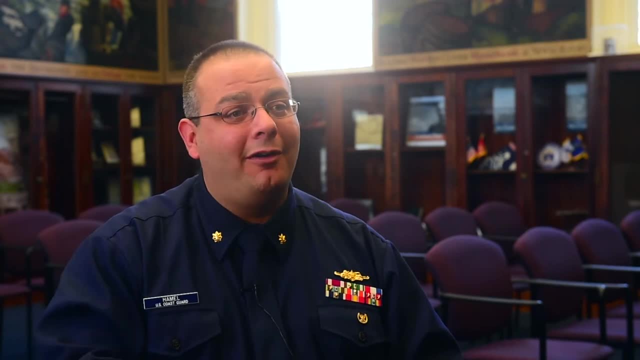 Whether you're an engineer or a management major, a government major, an OR or an MES, we're still driving that same goal through the core requirements: to give you a strong foundation and develop those traits that we want in the future leaders of the Coast Guard.